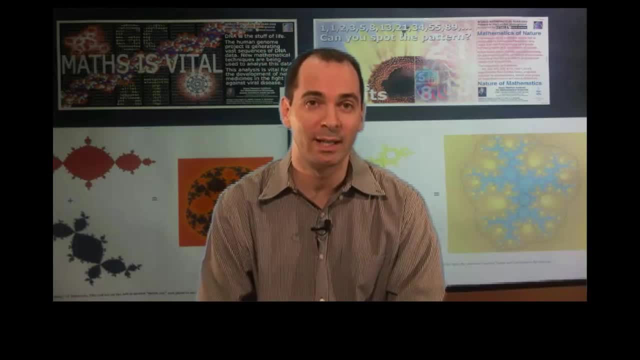 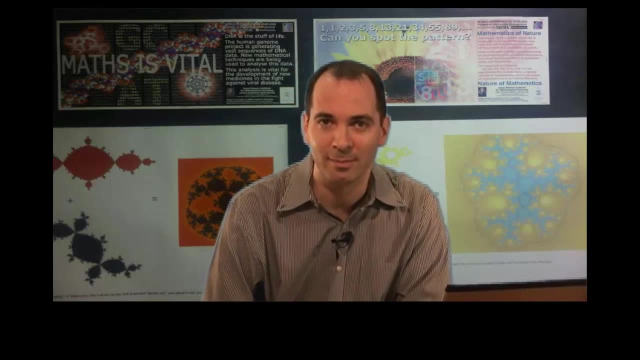 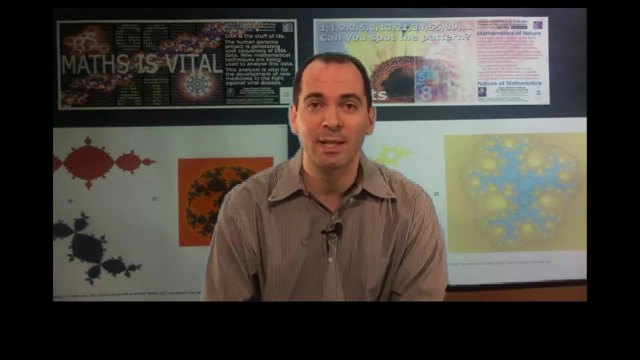 The definite integral, however, was motivated by the problem of finding the area of a plane region. At first, it seems like these two concepts are completely unrelated. After all, why would there be a connection between slopes of tangents and areas? Surprisingly, there is a deep and important fundamental connection between these two notions. 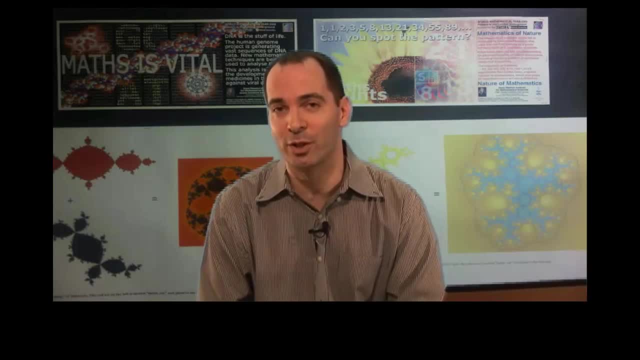 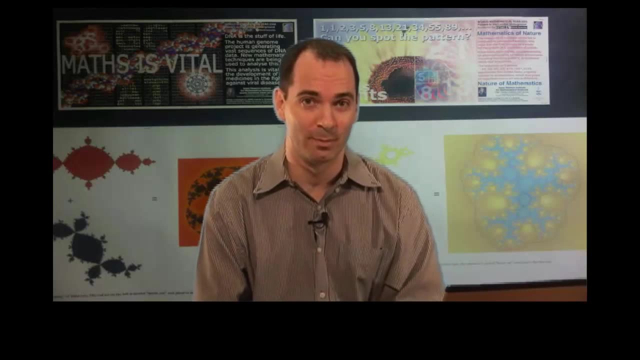 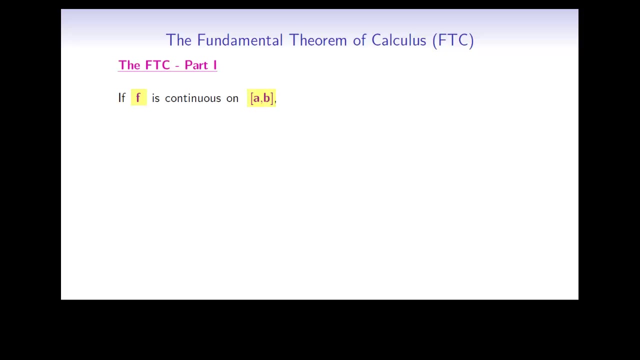 In some sense integration is the reverse operation of differentiation. This idea is made precise by the fundamental theorem of calculus. Here is the first part of the theorem: If f is continuous on the closed interval ab, then big F of x, given by the integral from a to x, of little f, of t, dt, is differentiable. 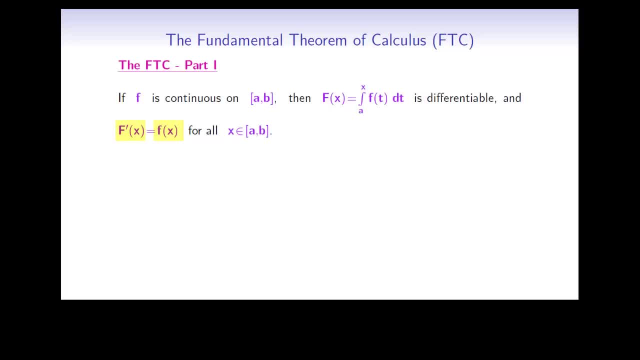 and big F. prime of x is equal to little f of x. for all x's in ab. This means that big F is an antiderivative of the function little f. Informally, this statement means that when you start with a continuous function, 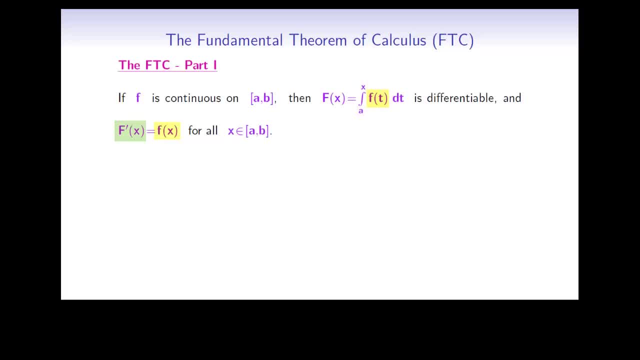 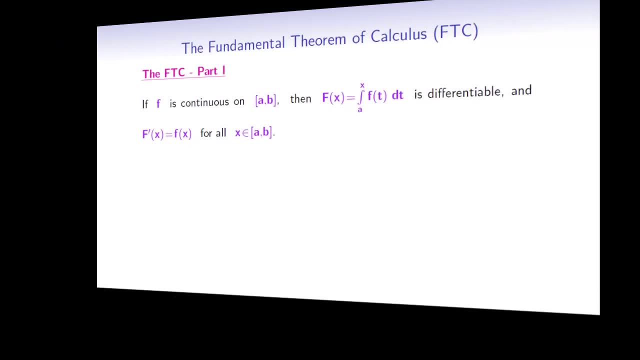 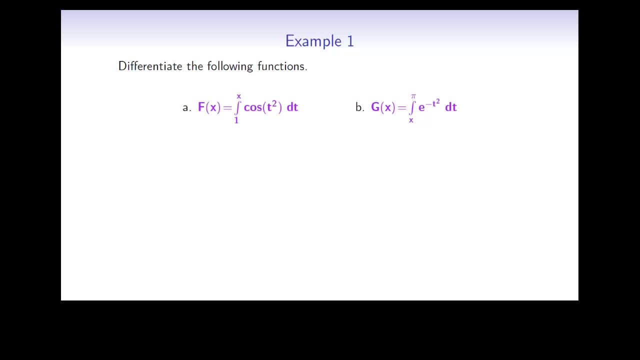 integrate it and then differentiate the integral, you get back your original function. Now let's have a look at a few examples. Differentiate the following two functions In part: the function big F is defined as the integral from 1 to x of cos, t2, dt. 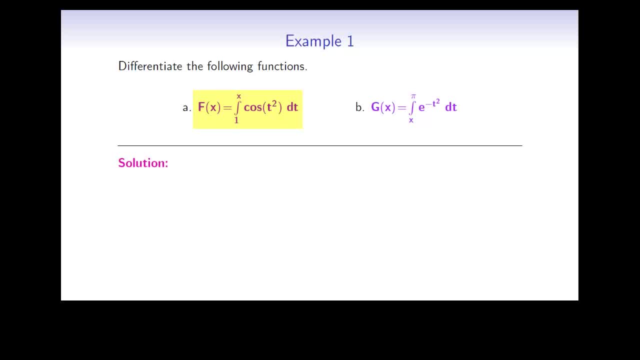 In this case we can apply the first part of the fundamental theorem right away, as the lower bound of the integral is a constant 1, and the upper bound is the variable x. So by the first part of the theorem we get that F prime of x is equal to cos of x square. 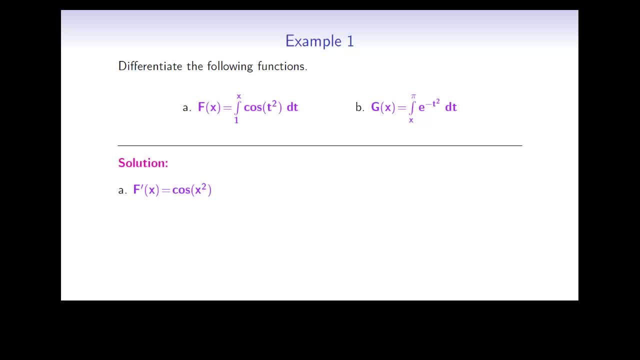 In the second part, in part, we have another function, g, of x, which is also defined as an integral, But this time the lower bound is the variable and the upper bound, pi, is a constant. So, before we use the first part of the fundamental theorem, 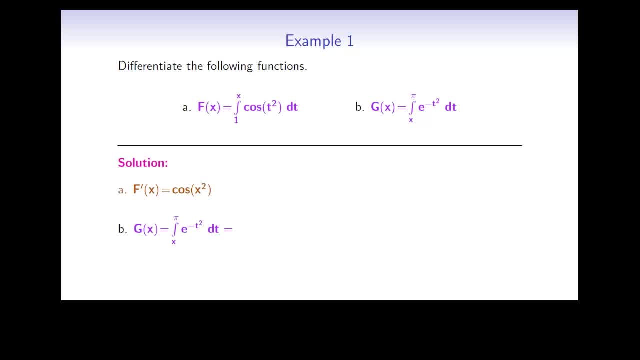 we will need to switch the order of the bounds. This would mean that we introduce a negative sign And now g of x is written as minus integral, from pi to x of e to the negative t square dt, and we can apply the first part of the theorem. 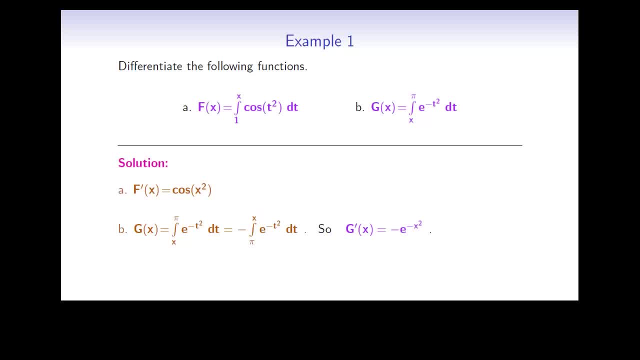 When we do that, we get g. prime of x is equal to negative e to the negative x square. Here is another example: Differentiate the function F of x, defined as the integral, from 1 to x squared of 1 over 2 plus cos t, dt. 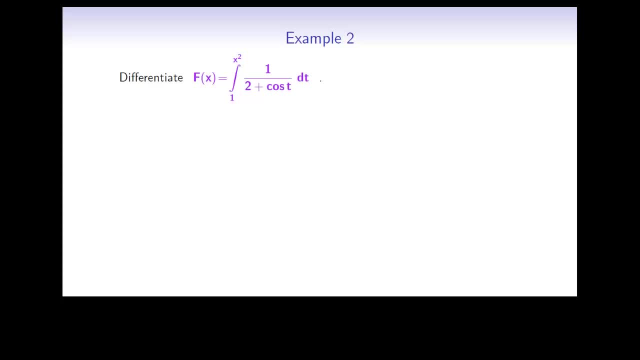 Here we have a function defined again as an integral. The lower bound is a constant number 1, and the upper bound is x squared, So we cannot apply directly the first part of the fundamental theorem. We can, however, do the following. 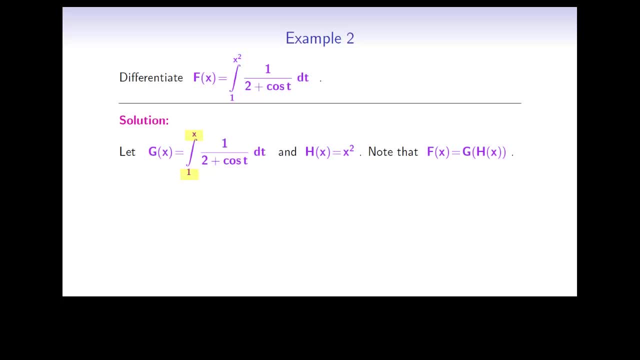 Let g of x be given by the integral from 1 to x of 1 over 2 plus cos t, dt, and let h of x be the function x squared. Note that g is almost the same as F. The only difference is that the upper bound 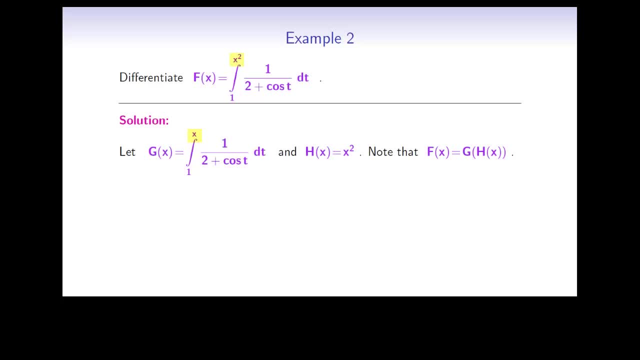 was taken to be x instead of x squared, so it will be easy to apply the first part of the fundamental theorem. Also, note that the composition g of h of x will be equal to the function F, because when you take the function g and replace x by x squared, 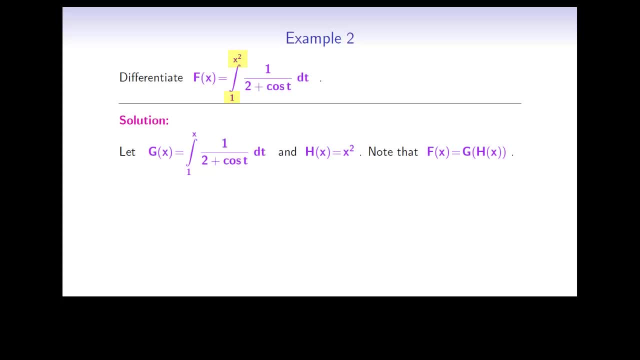 you get the integral that goes from 1 to x squared. Also, remember that the chain rule says that the derivative of a composition will be equal to g prime of h of x times h prime of x. g prime of h of x is equal to g prime of x squared. 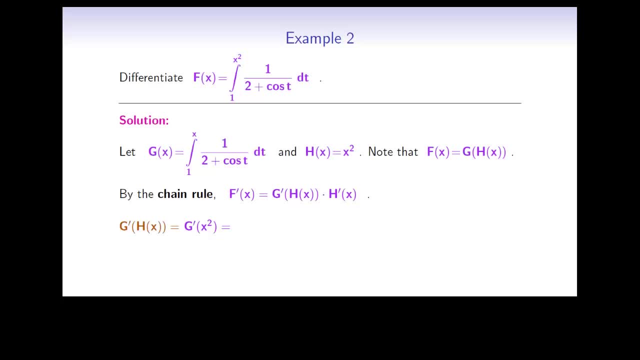 and now we can use the fundamental theorem to differentiate the function g. The derivative of g will be 1 over 2 plus cos x, and when evaluated at x squared, we get 1 over 2 plus cos of x squared. The derivative of h is very easy to compute. 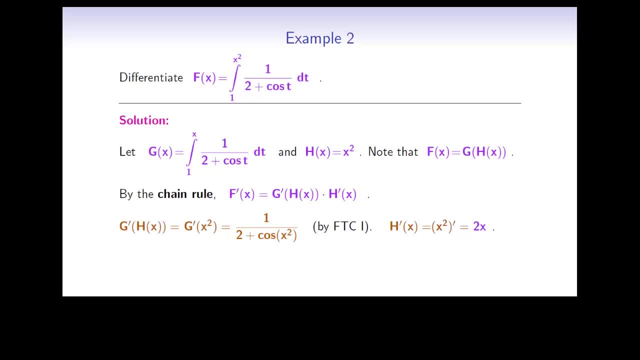 as x squared prime is known to be equal to 2x, And now all we need to do is multiply these two quantities and we get that F prime of x is equal to 2x divided by 2 plus cos of x squared. 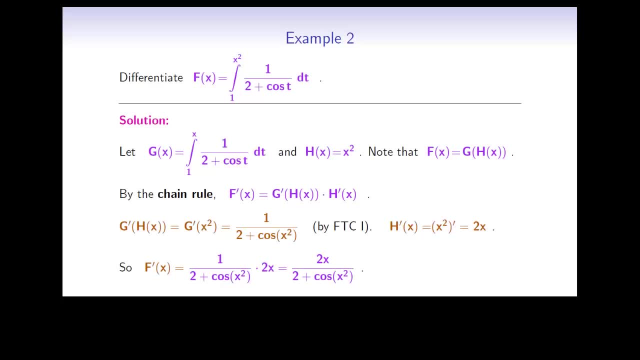 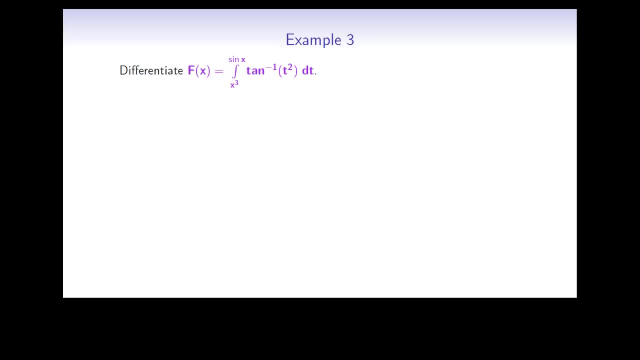 Now let's have a look at our last example of this type. Differentiate the function F of x, defined as the integral from x cubed, to sin x tan inverse of t squared dt. Here we have an integral in which both bounds are functions of x. 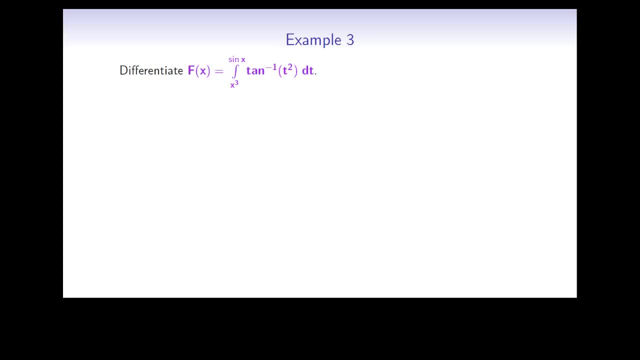 And so, before we differentiate F of x, we would like to write it as a sum of two integrals, each of which has a constant bound. So, using the basic properties of definite integrals, we can write the function F of x. 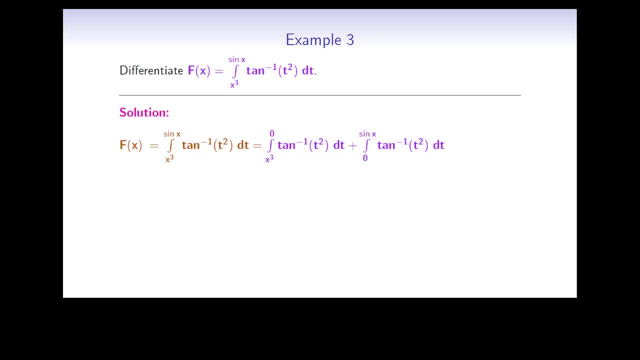 as the integral from x cubed to 0, of tan inverse t squared dt, plus the integral from 0 to sin x- tan inverse of t squared dt. We would also like our lower bounds to be constants, and so in the first integral. 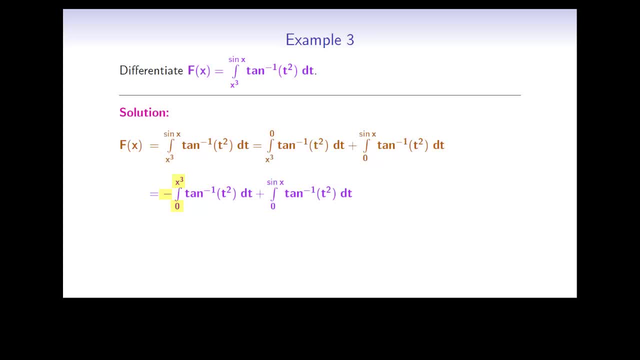 we will switch the two bounds and get negative integral from 0 to x cubed tan inverse of t squared dt, plus the integral from 0 to sin x tan inverse of t squared dt. Now we have two integrals and in each one of them, 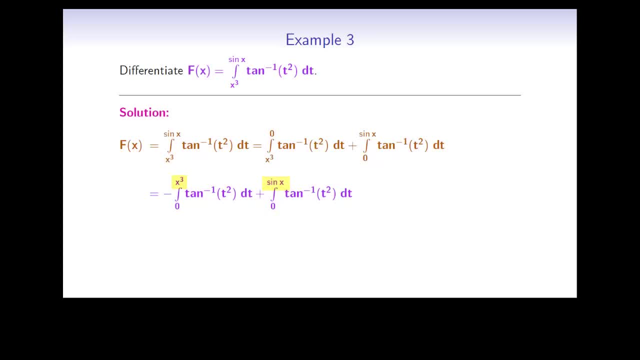 the lower bound is a constant 0, and the upper bound is a function of x, So we can apply the same method that we used in example 2, and differentiate these integrals. We will think of each of these integrals as a composition. 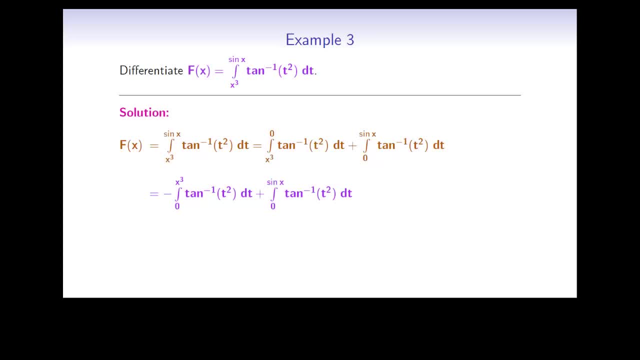 where the outer function is an integral that goes from 0 to x and the inner function is either x cubed or sin x, Then we will apply the chain rule to differentiate these compositions. We get the following: f prime of x will be equal to negative tan inverse of x to the sixth. 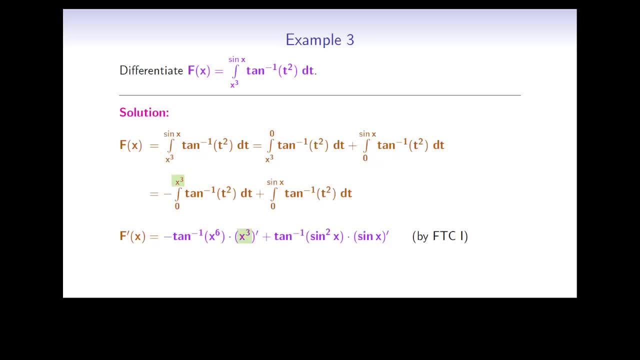 times x cubed prime. that's the derivative of the inner function plus tan inverse of sin square of x times again the derivative of the inner function: sin x prime. After computing these derivatives we get negative tan inverse of x to the sixth. 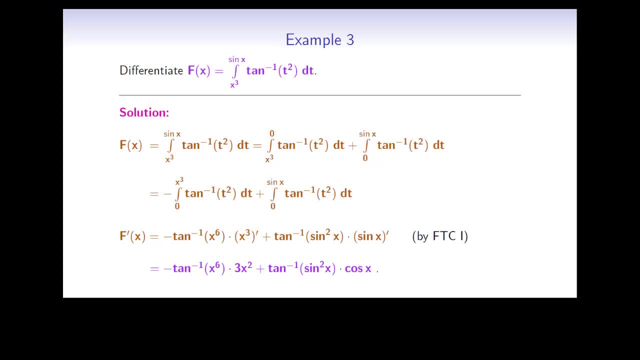 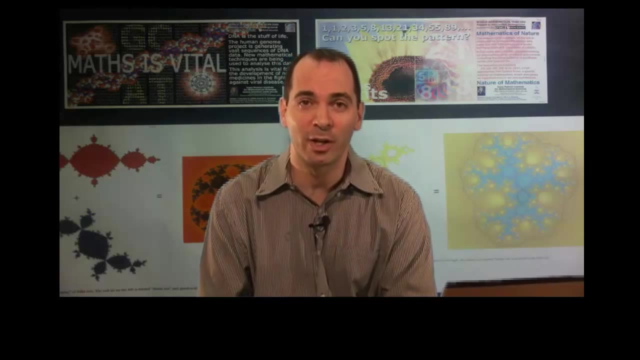 times 3x squared plus tan, inverse of sin squared x times cos x. So the first part of the fundamental theorem of calculus allows us to differentiate functions defined as an integral. The second part of the theorem, also called the evaluation theorem, 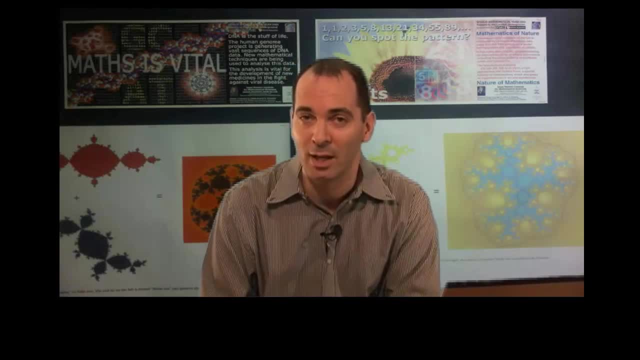 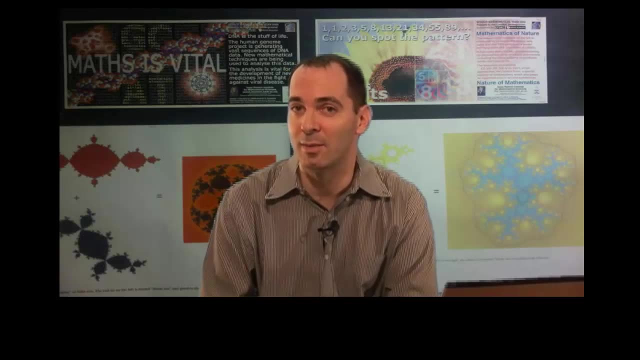 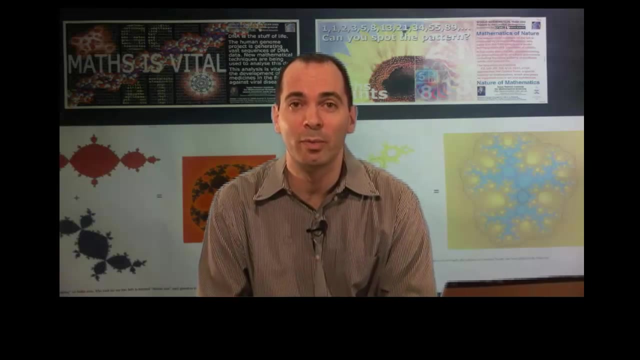 will be used to compute definite integrals. Recall that the definite integral of a function was defined as the limit of Riemann sums. But working with Riemann sums and finding their limits can be difficult and even impossible. in most cases, The evaluation theorem will be used to quickly evaluate. 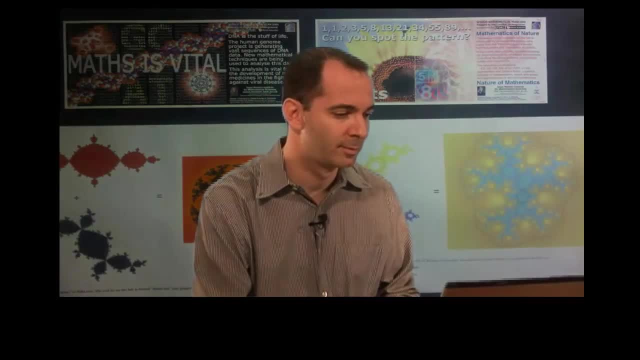 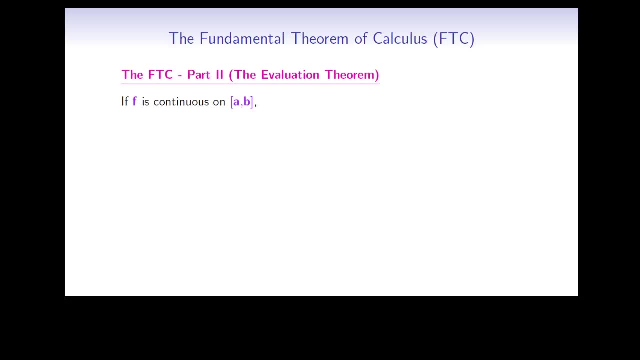 many definite integrals. The second part of the fundamental theorem of calculus says that if f is a continuous function on the closed interval ab and F is any antiderivative of f, then the integral from a to b of f dx is equal to F minus F. 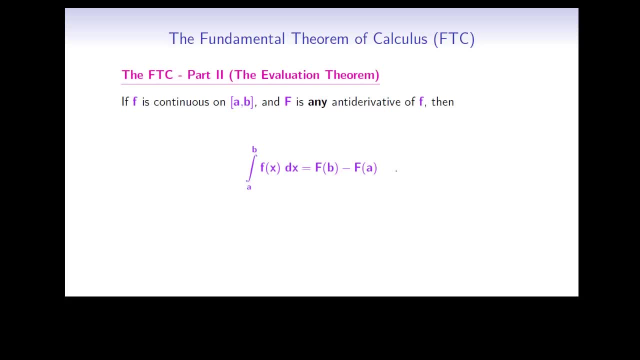 In other words, to compute a definite integral, it is enough to find one antiderivative of f, compute it at the endpoints a and b and then take the difference. Here is a remark: The notation f with a vertical bar, a at the bottom and b at the top. 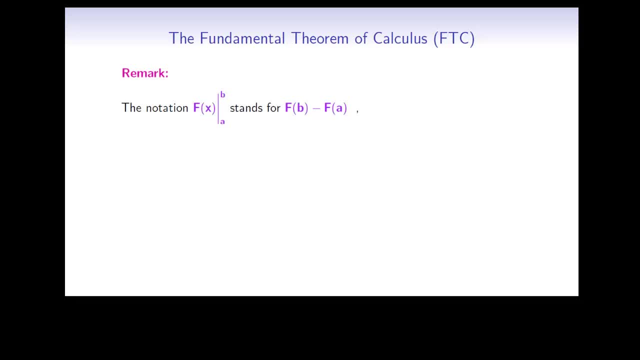 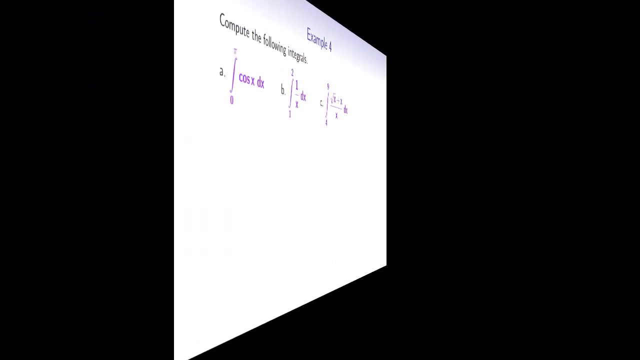 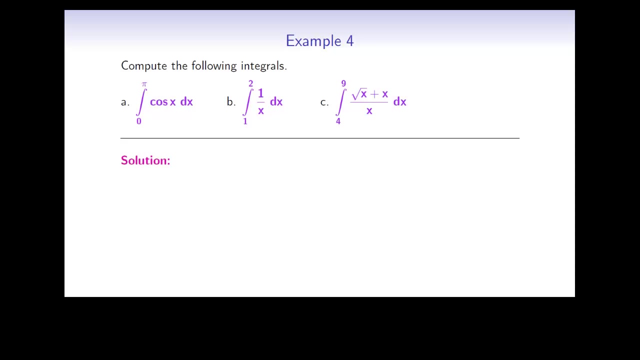 stands for the difference F minus F and will be often used when we work with the fundamental theorem of calculus. Now let's move on to some examples. Compute the following three definite integrals In part: we need to find the integral from 0 to pi. 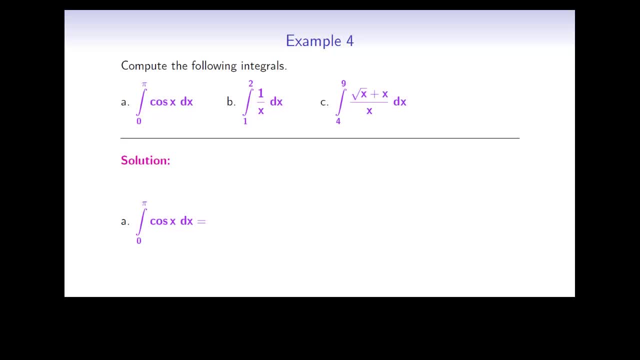 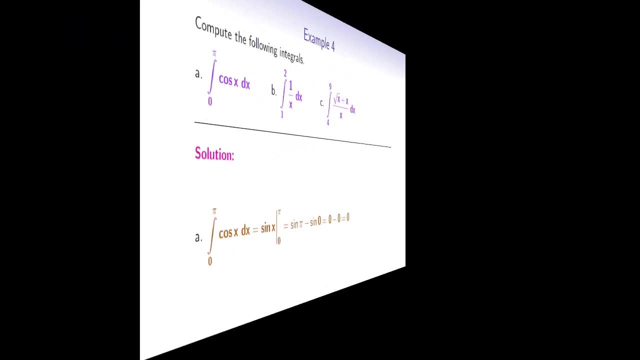 of the function cos. An antiderivative of cos is sin, and so by the fundamental theorem, we need to evaluate sin at pi and 0 and compute the difference. The final answer ends up being 0.. In part, we need to find the integral of 1 over x. 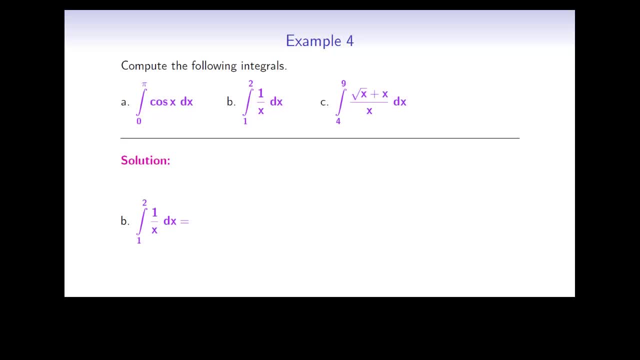 on the interval that goes from 1 to 2.. An antiderivative for 1 over x is ln, And so by the fundamental theorem we evaluate ln at the two endpoints and then compute the difference. We get ln minus ln, and as ln is equal to 0,. 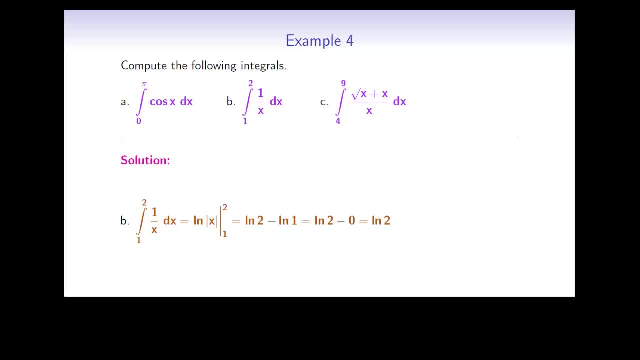 the final answer is ln. And finally, in part, we need to find the integral of square root of x plus x over x, from 4 to 9.. In this case, it would be better to first simplify the function and write this integral as the integral. 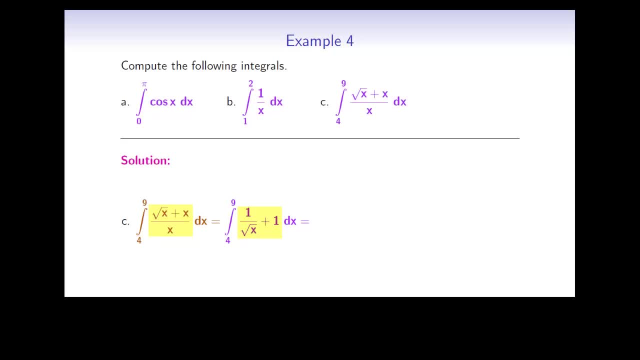 of 1 over square root of x plus 1 from 4 to 9 and then find an antiderivative. An antiderivative of 1 over square root of x is 2 times root x and an antiderivative for 1 is x. 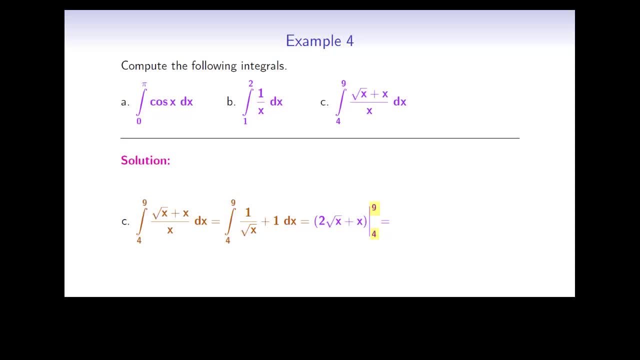 We evaluate this expression at 4 and 9 and then take the difference. We get 2 times 3 plus 9, minus 2 times 2 plus 4.. We get 15 minus 8, which is equal to 7, and that's the final answer for part. 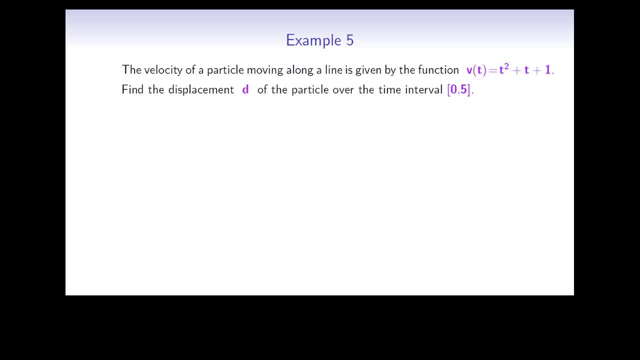 The last example in this video is of an applied nature. The velocity of a particle moving along a line is given by the function v of t, equals t squared plus t plus 1.. Find the displacement d of the particle over the time interval 0 to 5.. 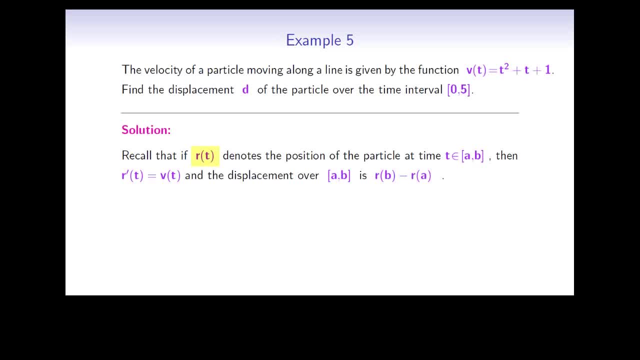 First let's recall that if r of t denotes the position of the particle at time t, then the derivative r prime of t will be the velocity of the particle at that time And the displacement over a time interval. ab is the difference r of b minus r of a. 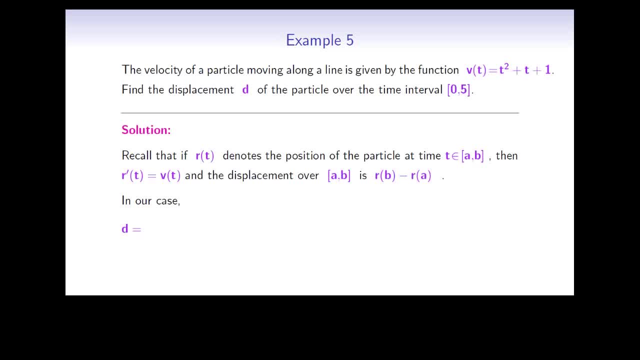 In our case we need to find the displacement over the time interval 0 to 5.. So d will be equal to r of 5 minus r of 0.. This difference can be also written using the vertical bar notation, According to the fundamental theorem.